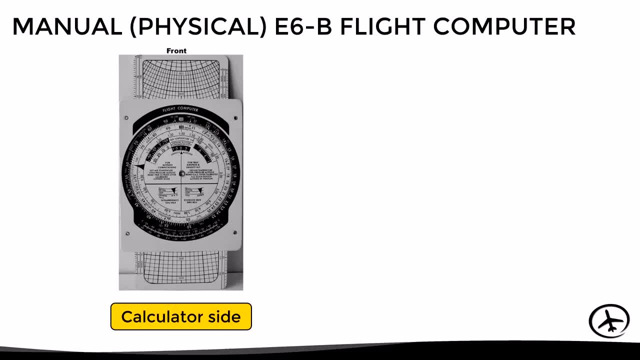 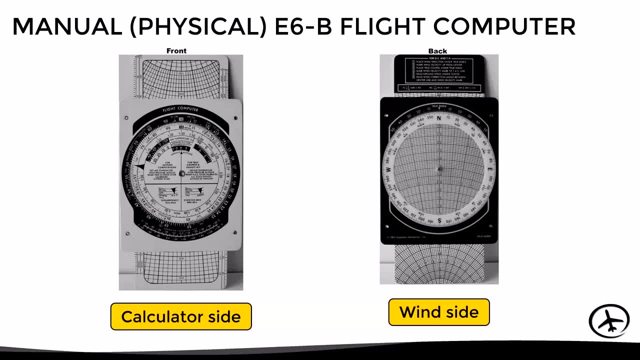 two sides: the calculator, or front side, which we talked about in detail in the previous video, and the wind, or back side, which we will focus on in this video. With this being said, the wind side consists of a transparent rotating disc with the compass. 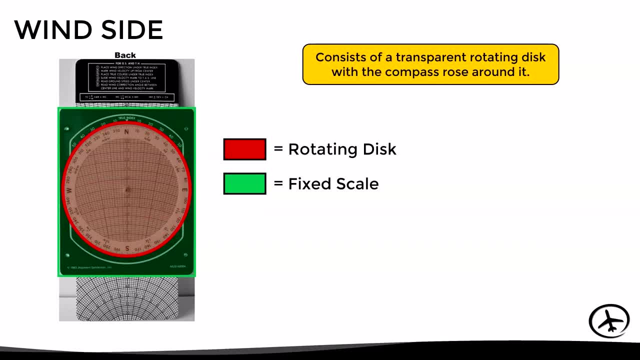 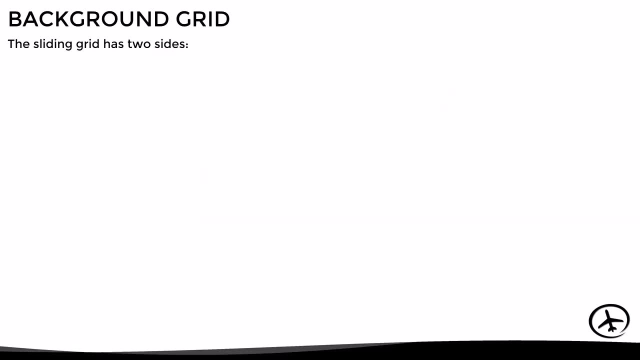 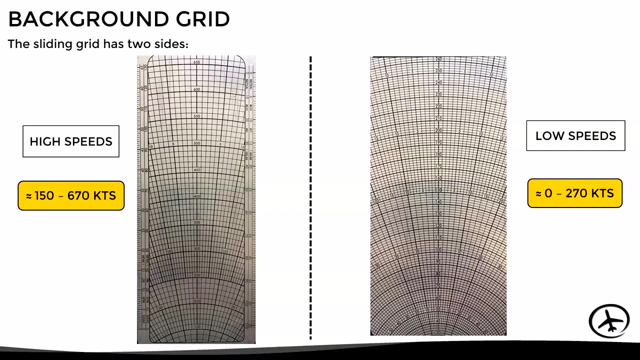 rows around it, Which, in turn, is inside a fixed scale that can be moved along a background sliding grid. Now, this background grid also has two sides, one of them used for high speed calculations and the other one used for lower speeds, So the grid to be used will depend on the problem we are solving. 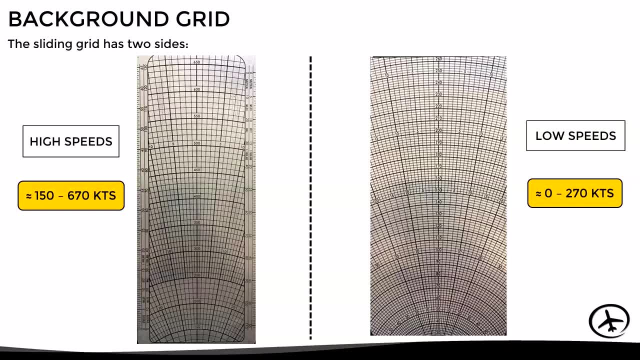 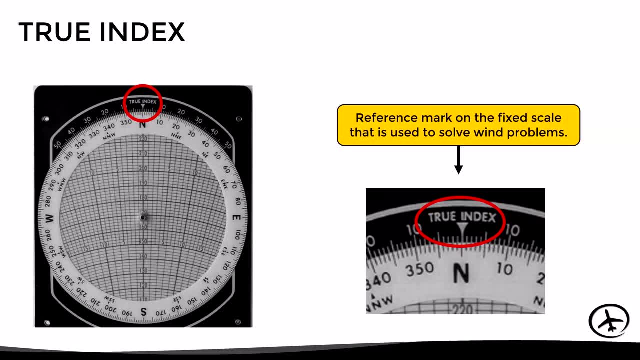 With this in mind, let's look at the different reference markings that we can find in the wind side of the flight computer. One of the most important ones is the true index. This is the reference mark on the fixed scale, as we can see in this images. 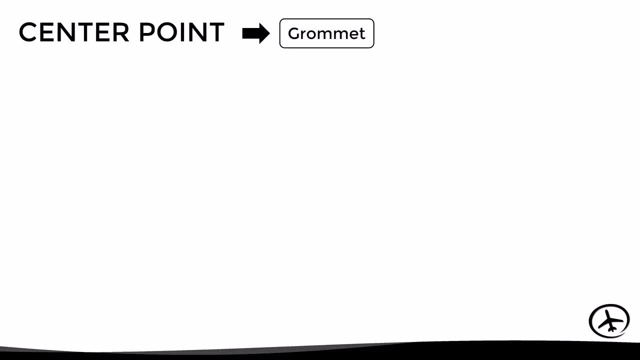 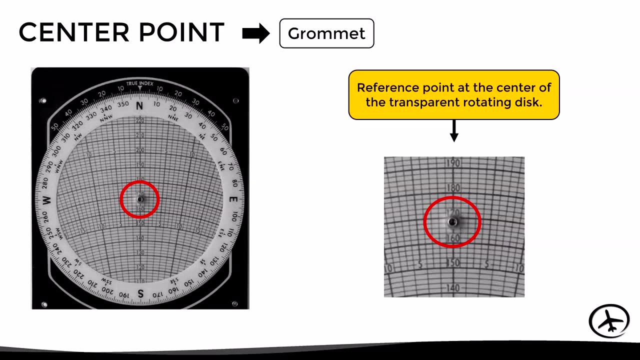 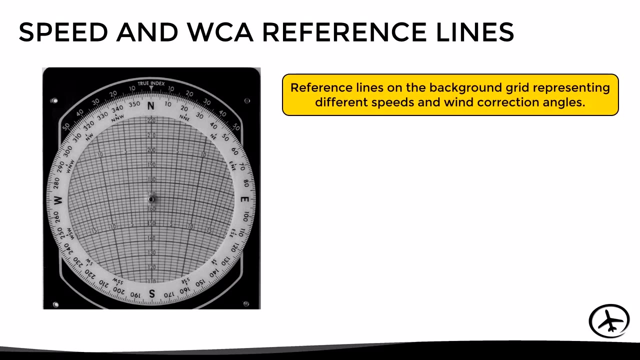 Other important mark is the center point, also known as grommet, which is a reference point at the center of the transparent rotating disc. And finally, there are the speed and wind correction lines, which are located on the background sliding grid, representing different speeds and wind correction angles. 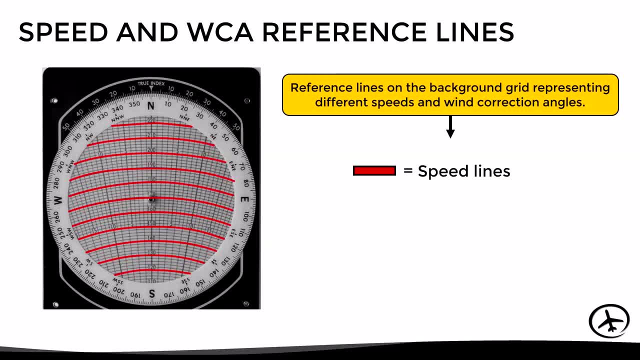 In this example, the transverse red lines represent the speed, The red lines represent the speed of the flight, The red lines represent the speed of the flight, The red lines represent the speed of the flight And the longitudinal yellow lines represent different wind correction angles. 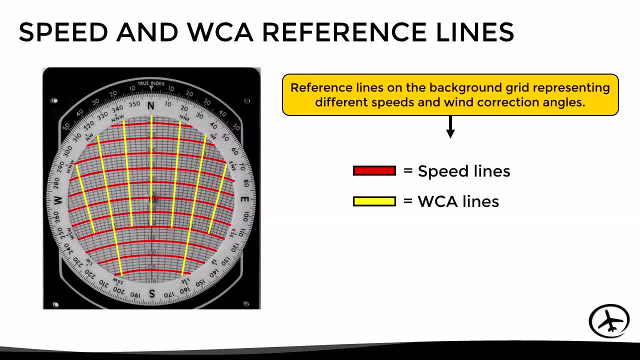 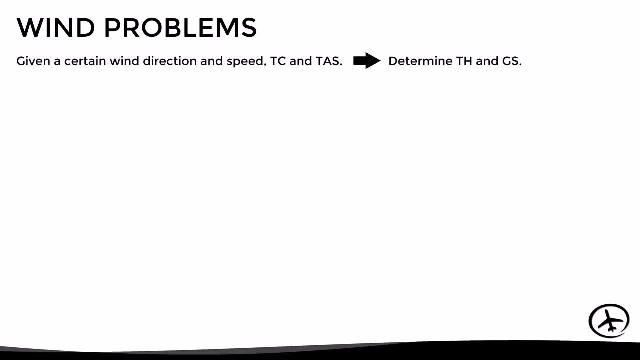 So, having already seen the most relevant parts of the wind side, let's see how to solve one of the most common wind problems in navigation. and it is given a certain wind direction and speed, true course and true airspeed determine the true heading and the ground speed. 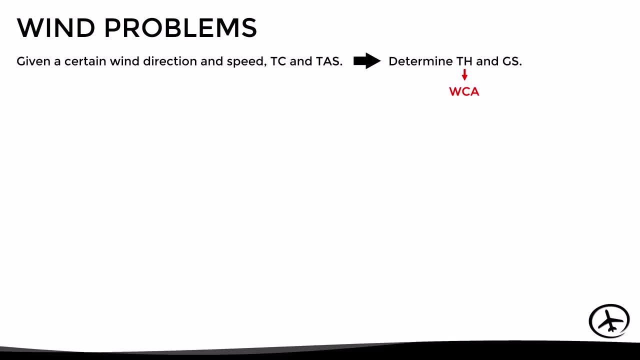 In other words, we have to calculate how is the aircraft going to be affected, in terms of track and speed, by the effect of wind. So to solve this problem, we have to follow these steps. First of all, align the wind direction with the true compass. 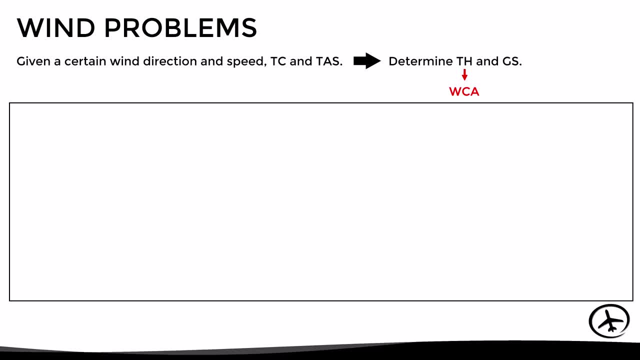 Then adjust the grommet on the 100 knot line or any other speed reference line that we to wish, Then make a mark with a pen or a marker that represents the current wind speed measured from the reference line where the grommet is located. 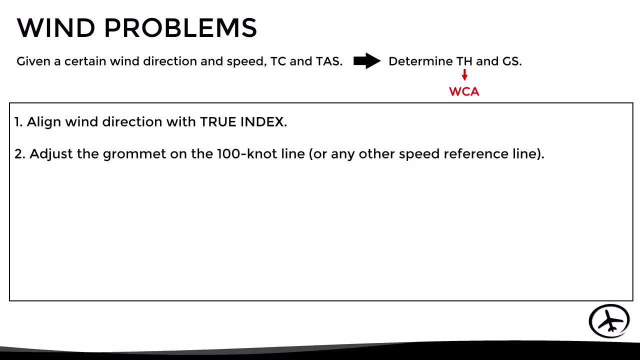 Then rotate the disc to align the true course with the true index and move the control wheel to align theいただ. having failure, This means there's no point in staying in the position of theOOK solution and volume 1.. Now that we've answered all the questions, we can increase the speed to 200 nautical. 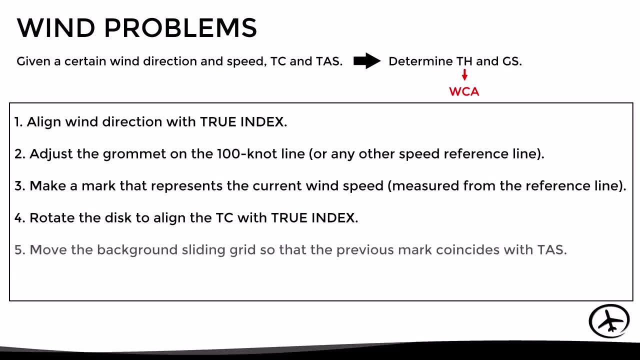 perché. And now we canaten Once a turn. Now ask if You want to Angle the course You would like to play it on by the index and move the background sliding grid so that the mark that we made coincides with the true air. 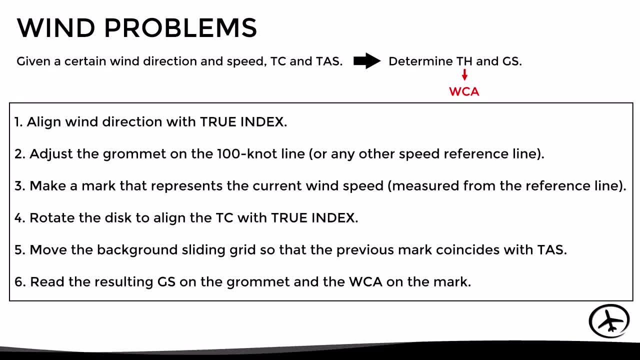 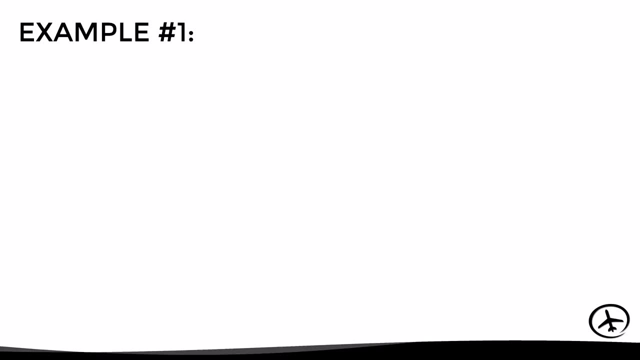 speed And finally read the resulting ground speed on the grommet and the wind correction angle on the mark. Now this may sound a bit complex and confusing, so let's look at this through an example. In this case, we have to determine the wind correction angle- true heading. 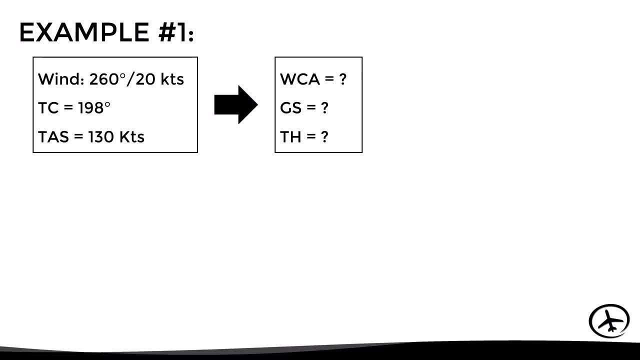 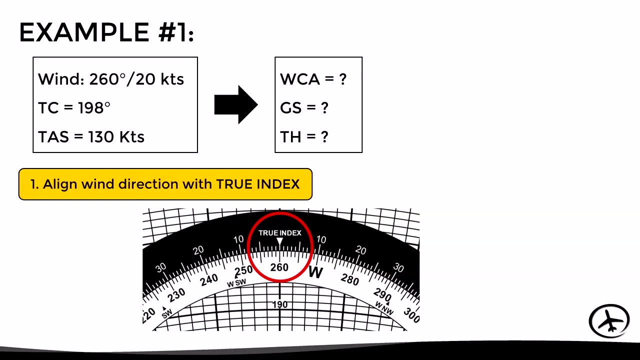 and ground speed, given a wind of 260 degrees at 20 knots, a true course of 198 degrees and a true airspeed of 130 knots. So let's do this step by step. First, we have to align the wind direction- which in this case is 260, with the true index, as we can see in this image. 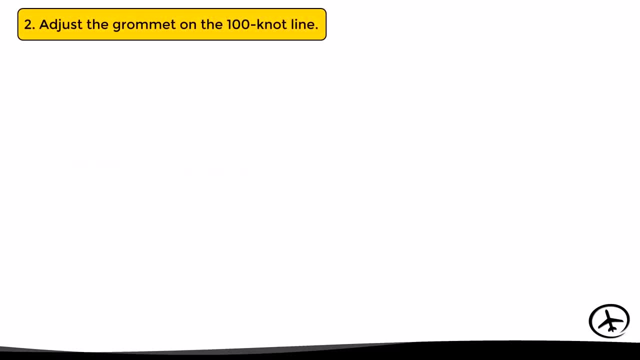 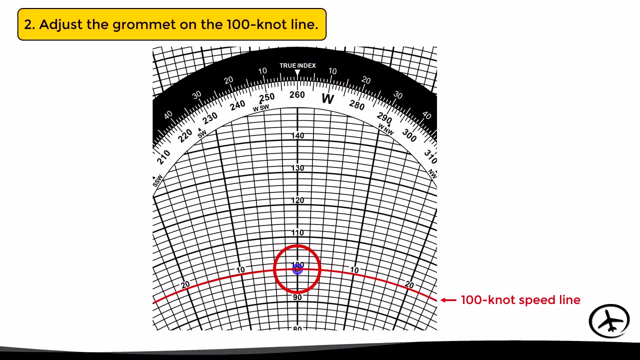 Once this is done, the second step is to adjust the grommet on the 100 knot line. This is a grommet that we will use to adjust the grommet on the 100 knot line. This is accomplished by moving the background sliding grid until the 100 knot line coincides. 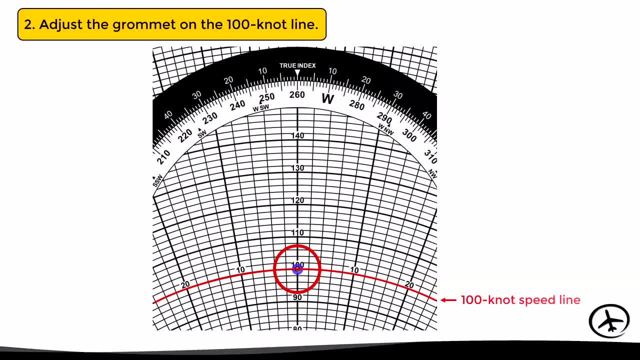 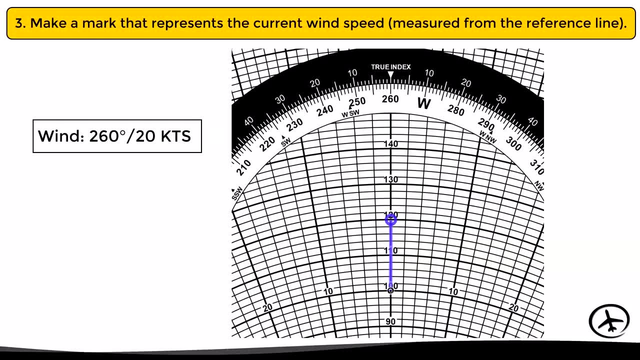 with the grommet. Then, using this line as reference, we have to make a mark that represents the current wind speed. In this case, since the wind speed is 20 knots and we are using the 100 knot line as reference, we have to make a mark at the 120 knot line, directly above the grommet. 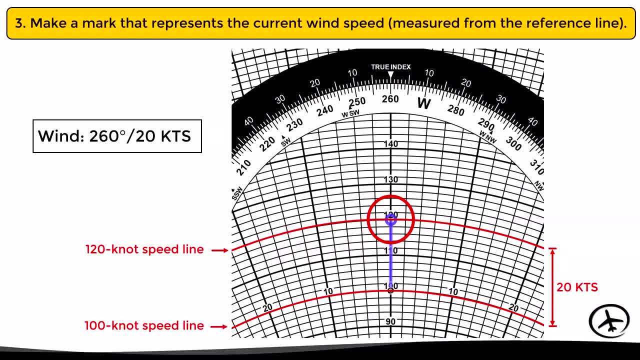 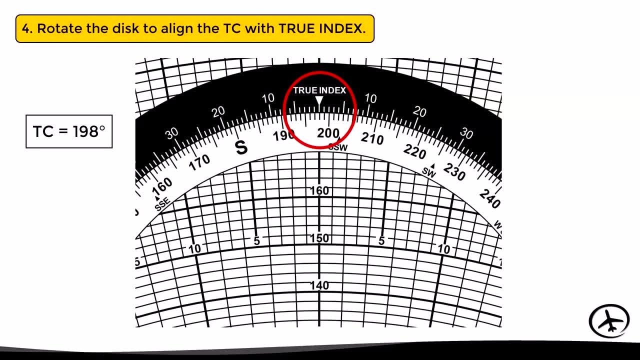 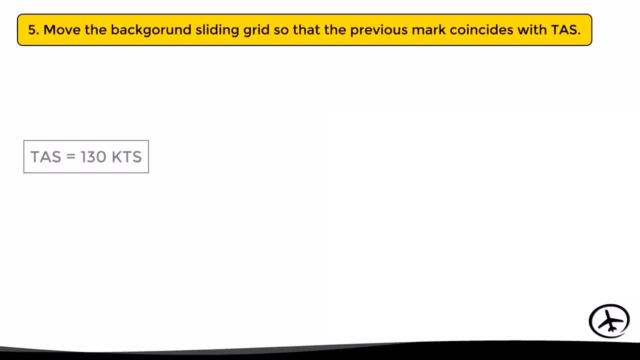 as we can see in this image. Once this mark is made, we have to rotate the disc to align the true course- which in this case is 198, with the true index. Then we move the background sliding grid so that the mark that we made coincides. 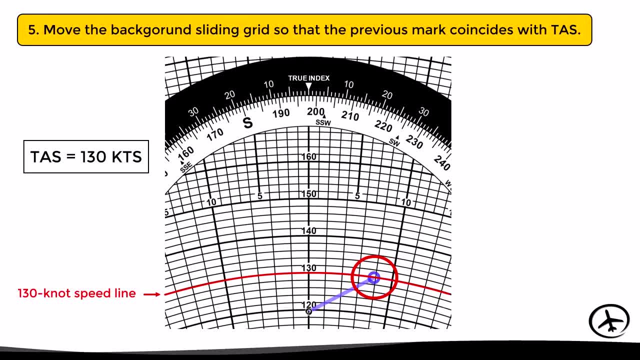 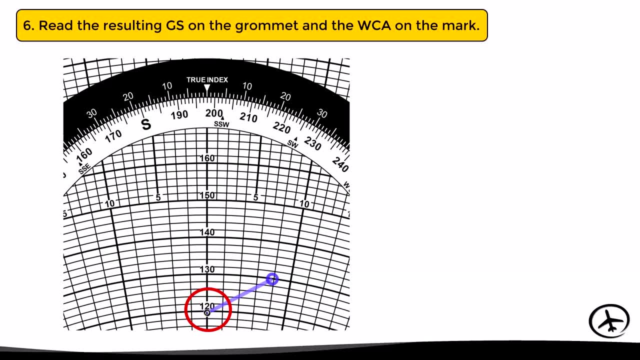 with the true airspeed, which in this case is 130 knots. Finally, with this configuration, all we have to do is read the resulting ground speed on the grommet, which in this case is 119 knots, and the wind correction angle on the mark. 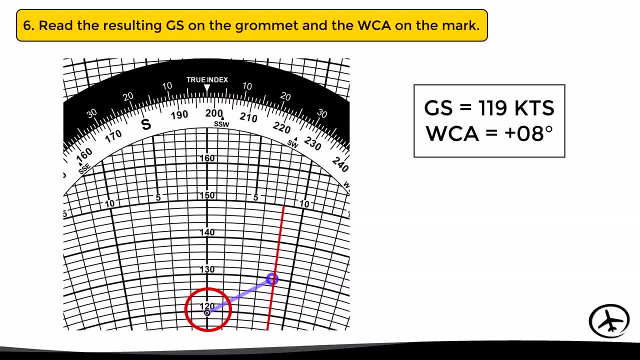 Here, all wind correction lines to the right of the grommet will be positive, while the ones to the left will be negative. With this, the wind correction angle would be plus 8 degrees. Now, with this information, we just have to take the true course and add. 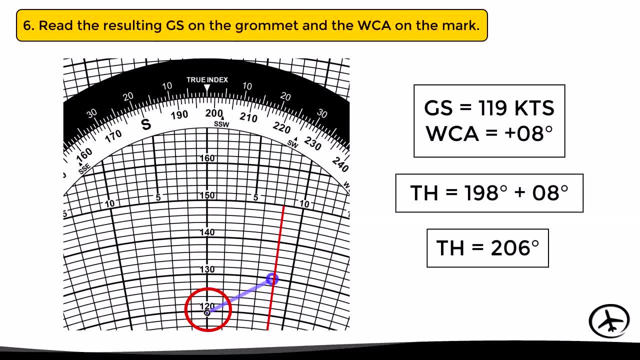 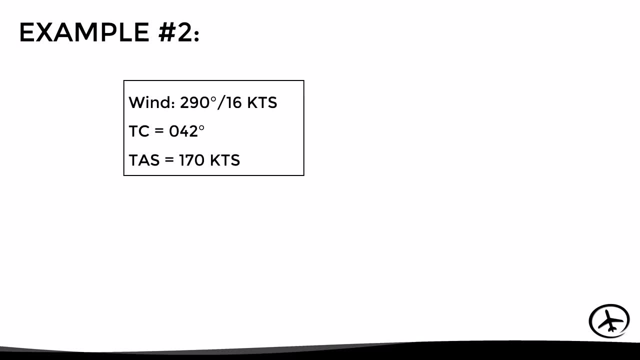 the wind correction angle to obtain a true heading of 206 degrees. If the procedure is not clear yet, let's take a look at another configuration For this example. we will assume a wind of 290 degrees at 16 knots, a true course of 042 degrees. 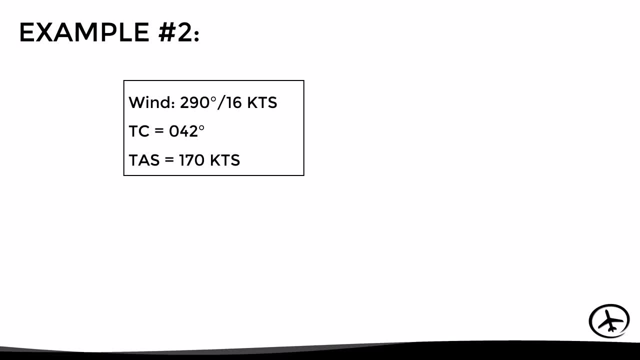 and a true airspeed of 170 knots. So, again based on this information, we have to determine the wind correction angle, the true heading and the ground speed. So, as mentioned earlier, the first step is to align the wind direction with the grommet. 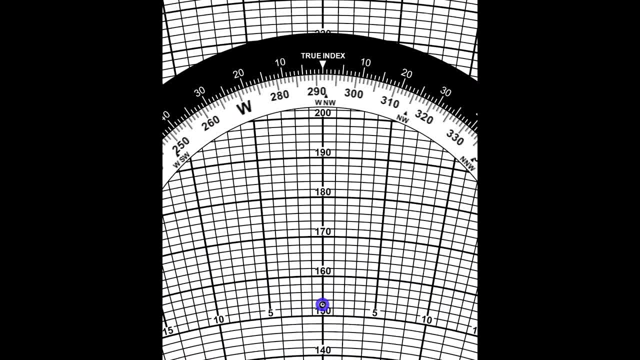 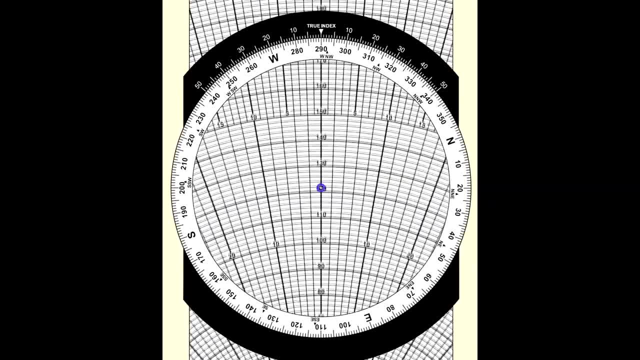 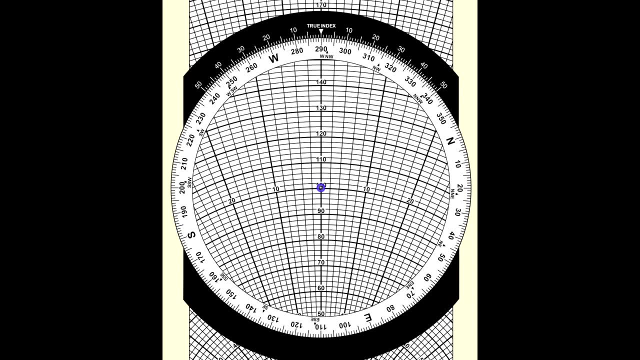 with a true index, which in this case is 290.. Then we move the background sliding grid to align the grommet with the 100 knot line. Then, using this line as reference, we make a mark on the transparent disc that represents the current wind speed, which in this case is 16 knots. 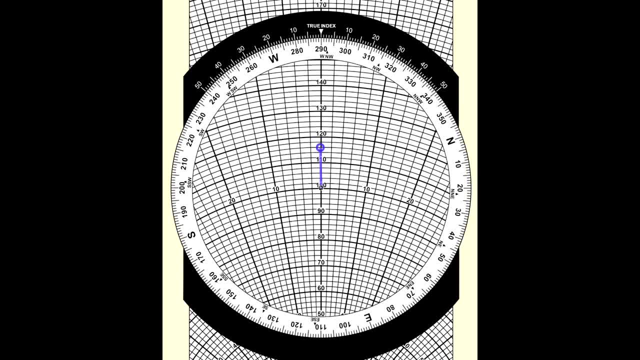 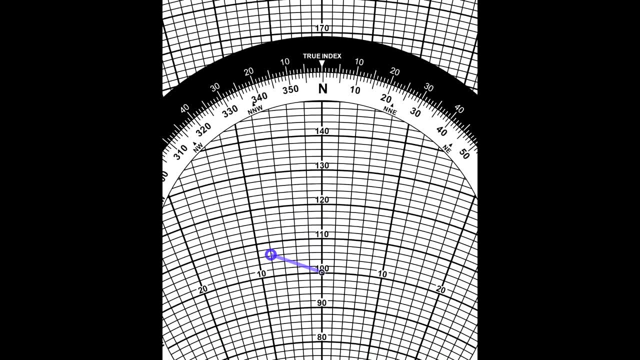 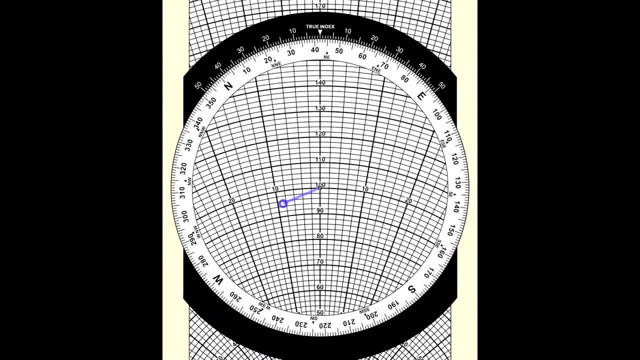 so we make the mark on the 116 knot line directly above the grommet. We turn the disc to align the true course with the true index, which in this case is 042.. After doing this, we move the background sliding grid so that the mark coincides. 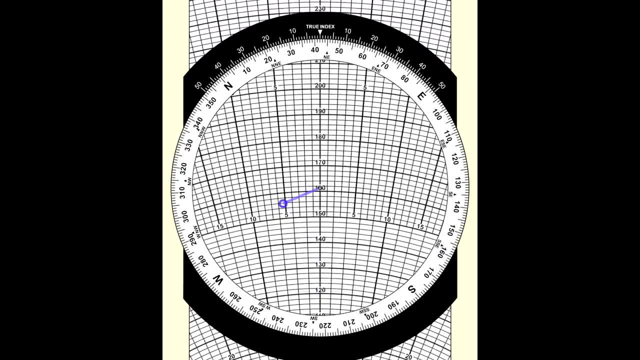 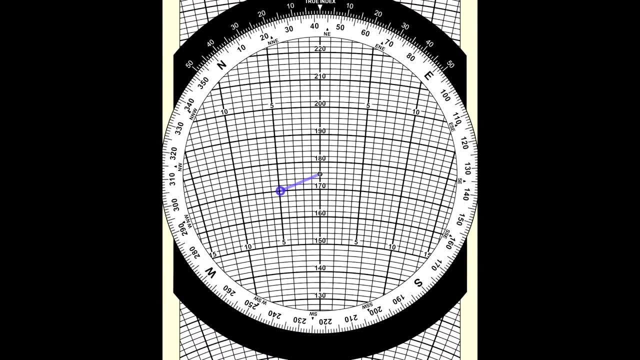 with the true airspeed, which in this case is 170 knots. Once this is done, we just read the ground speed on the grommet, which is around 175 knots, and the wind correction angle on the mark, which is on the 5 degree line. 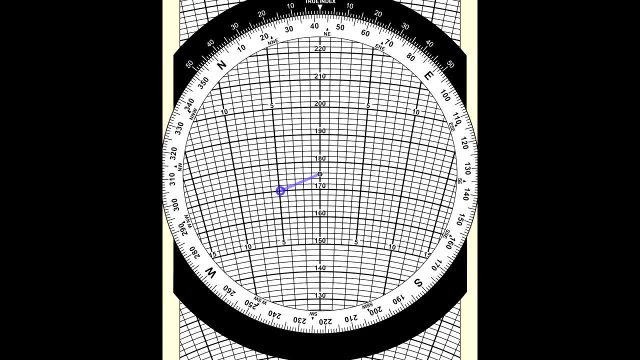 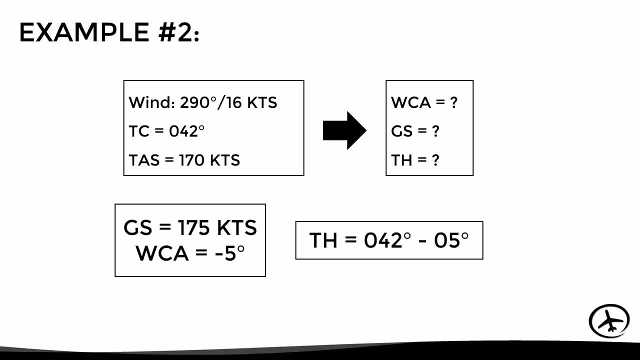 And finally, with this information, we just have to add the wind correction angle to the true course to obtain the true heading of 038.. And basically this is the way to proceed with any practical wind problem using a manual or physical flight computer. so it is important to practice a lot with several problems to